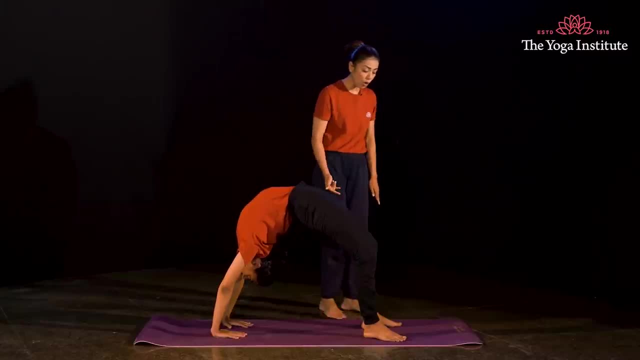 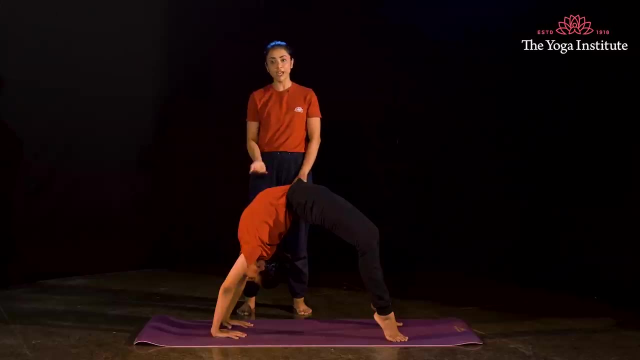 You are pressing grounding into the mat through your feet, Pressing the corners of your feet firmly into the floor. Your toes are parallel to each other. From here raise the heels up, trying to elongate the arch of your back. Your tailbone is pointing towards the knees. 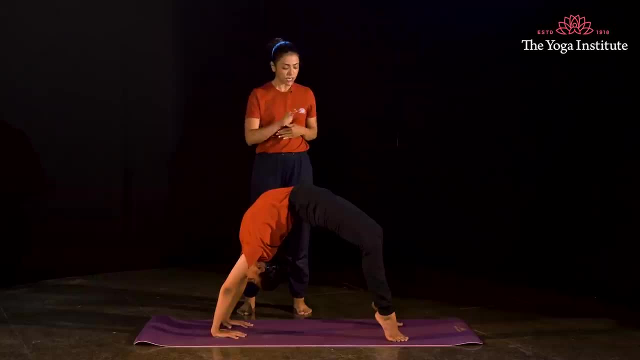 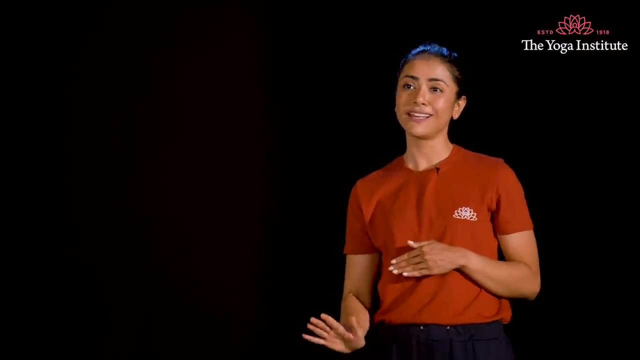 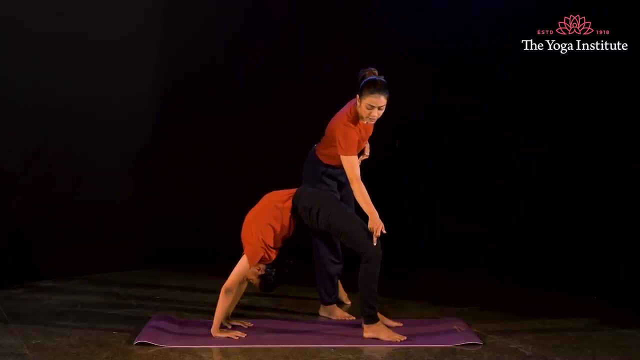 Maintaining this arch, this U shape of the body. you gently bring the heels back down, Just inhale and exhale here, staying in this posture for at least half a minute or a minute. Your knees are just above the heels. Your knees are not flaring out parallel to each other. 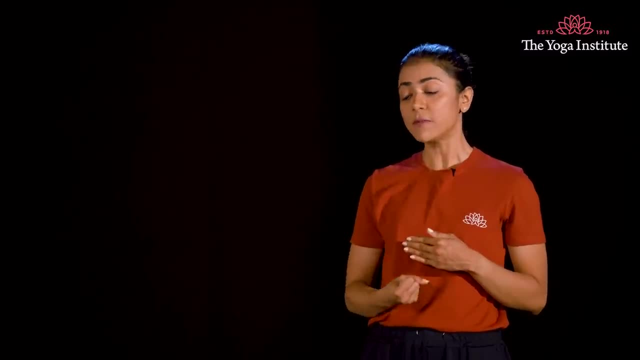 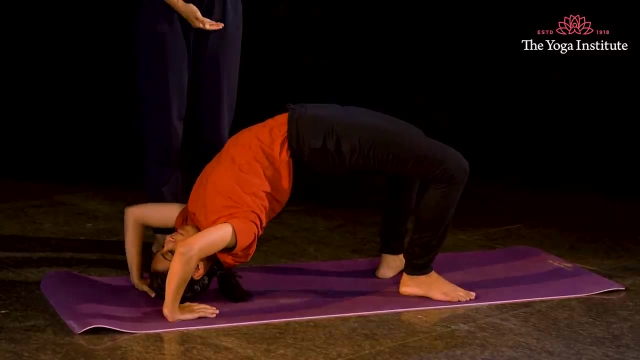 Engaging the abdomen. core is engaged. abdomen is tout. Now to come out of the pose. bring the top of the head on the floor, lowering down your hips and adjusting the upper chest, Lying down completely on the back again. 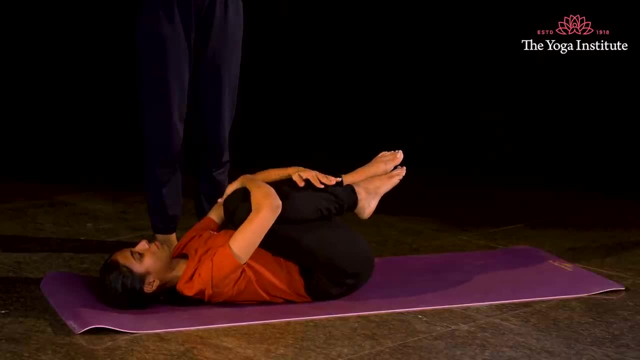 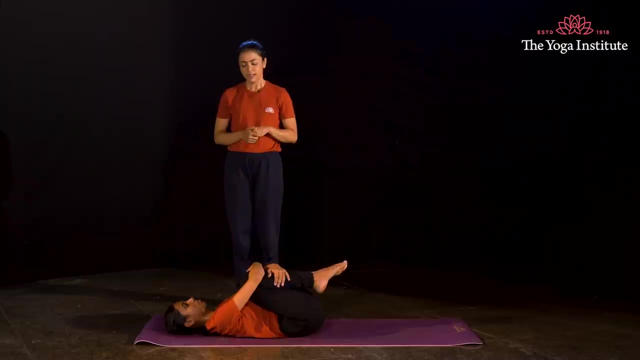 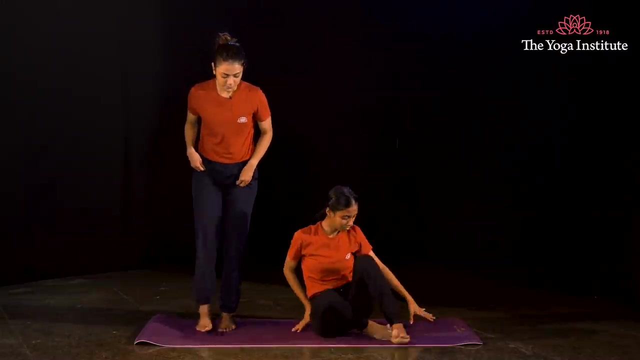 Now bring your knees closer to the chest, hugging your knees to your body, and roll side to side, massaging your lower back. This is how you end the posture. So now Hansa Maa will give us deeper insights about this asana. 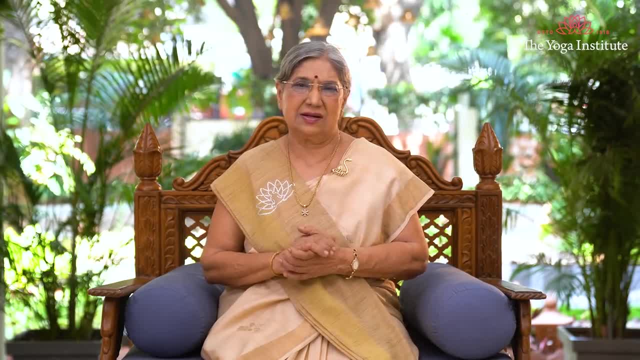 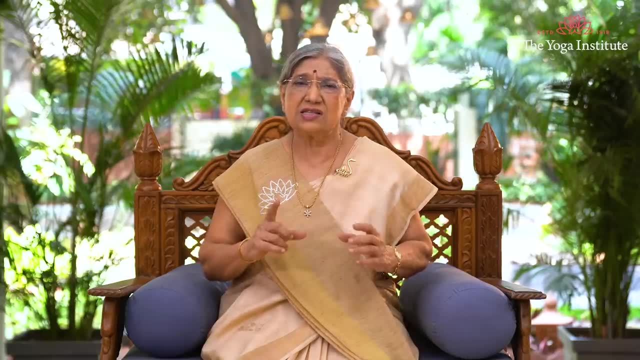 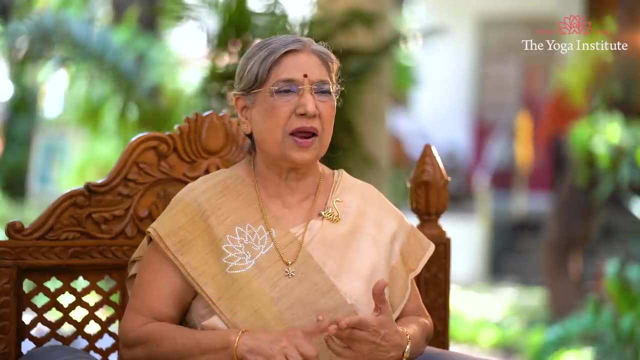 Chakra asana is a very intense and powerful asana. It can improve the balance of your mind and really induce self-confidence. So you understand, the dynamics of this asana are so wide and hence this asana should be practiced with utter focus. 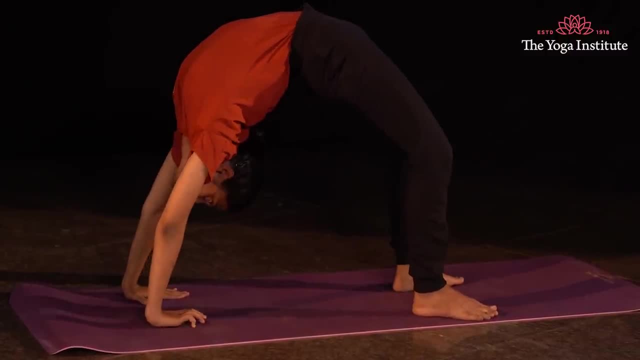 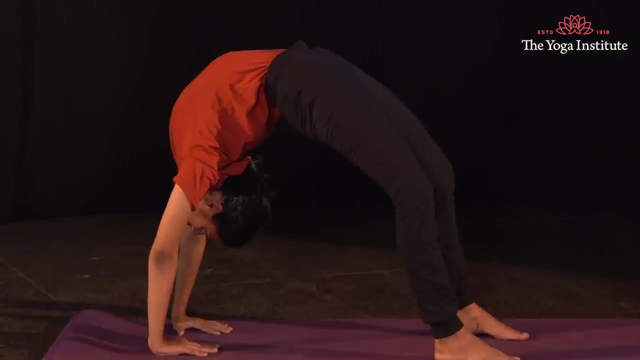 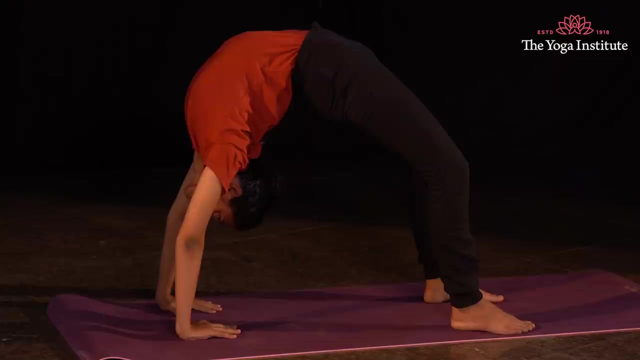 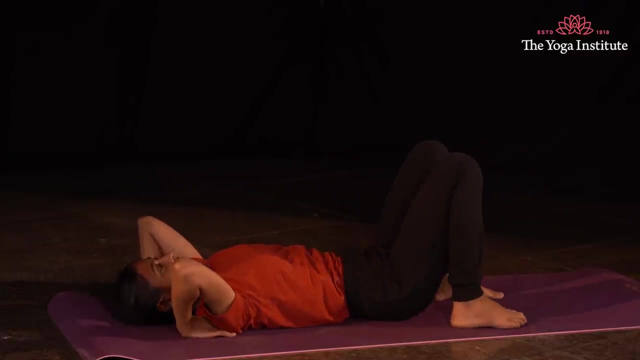 The movement of lifting body against gravity towards the sky generates a sense of Aishwarya Bhava, that is, self-confidence in life. Lift yourself with the thought of rising above all the challenges. It also involves the letting go factor. You cannot go down unless you let go of your lifted body to reach to the starting position. 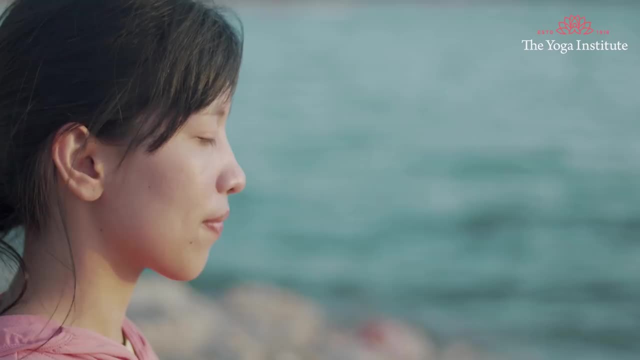 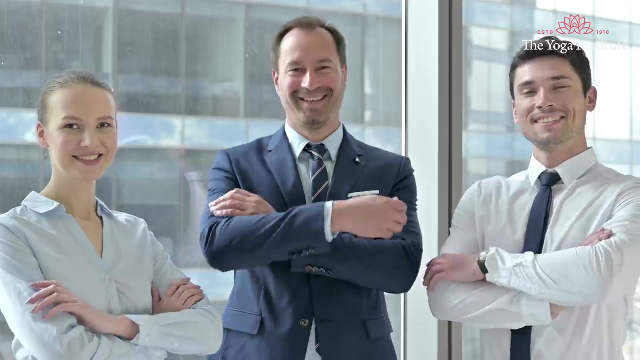 These skills that you acquire, you will be able to achieve. These skills that you acquire during the practice imprint themselves on your mind and you may observe the same attitude of letting go and confidence in all your activities throughout the day. Keep practicing this asana. 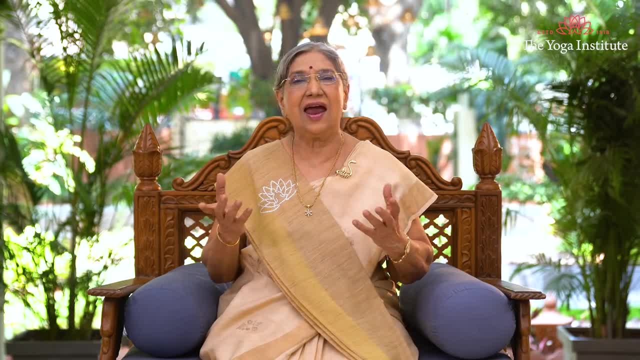 You will see huge difference, physically and mentally, Namaskar.